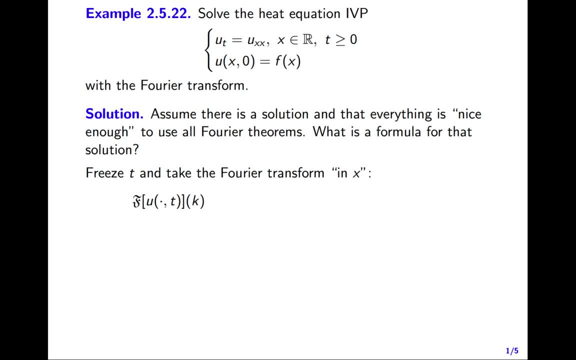 is only given for t greater than or equal to zero, whereas space x is given for all real numbers. And the Fourier transform requires us to integrate from minus infinity to infinity, And the only thing going from minus infinity to infinity here is x. So I'm going to take the 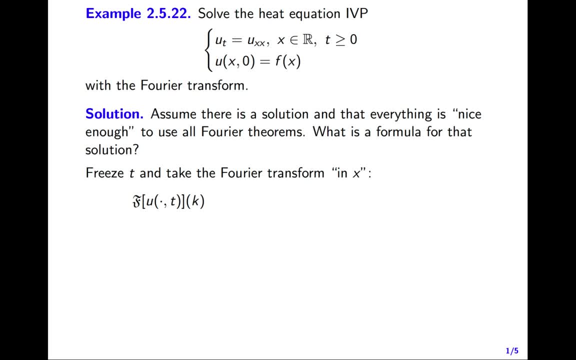 Fourier transform in x Fourier transform on u of dot t at k. What do I mean by that notation? I've frozen t, that's why t is a parameter. the x slot I've replaced with a dot to indicate that that is the independent variable of the function inside the Fourier transform and I'm evaluating. 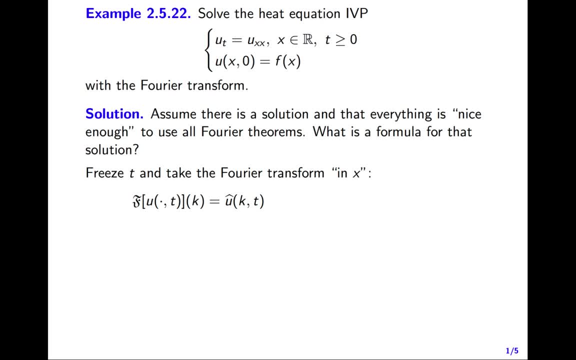 that at k And specifically, or I'll write that as u hat, of kt, and that will be the integral from minus infinity to infinity of u, of xt, e to the minus ik, x, dx times the usual 1 over root, 2, pi. So look at this integral. 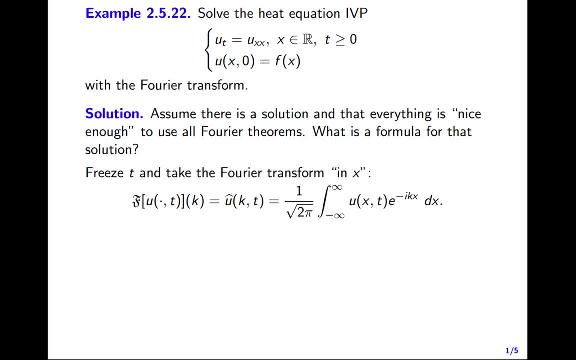 It's similar to what happened when we took Fourier coefficients for a function of two variables back in Fourier series. land. I have my usual 1 over root, 2, pi- I have the improper integral I'm integrating here with respect to x. so x appears three times as the dummy variable of. 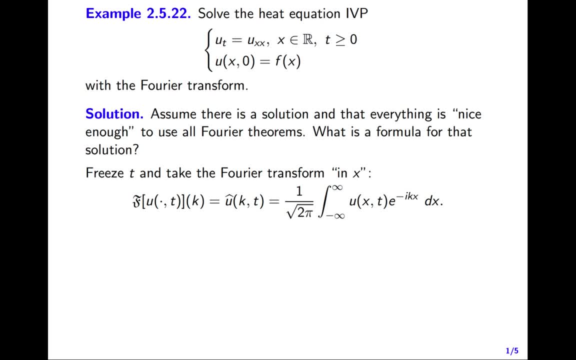 integration. t is now a parameter that's just coming along for the ride inside the integral and then in this e to the minus, ik, x, x is the dummy variable and k is the Fourier variable. So u hat of kt. the only things in this integral that can move are the k parameter. 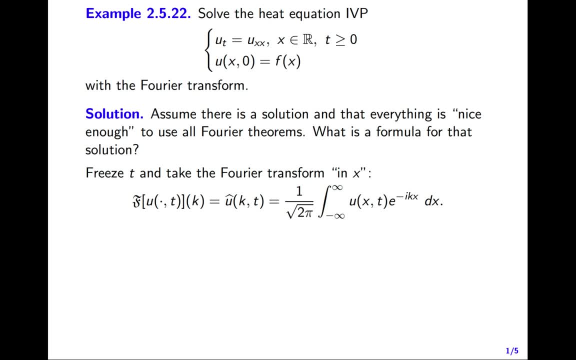 the Fourier parameter and the t parameter. the time parameter x is now completely gone. I could write w, I could write theta instead of x Inside this integral, it doesn't matter. And then if I do the transform of the x derivative for a transform on uxx dot t at k. 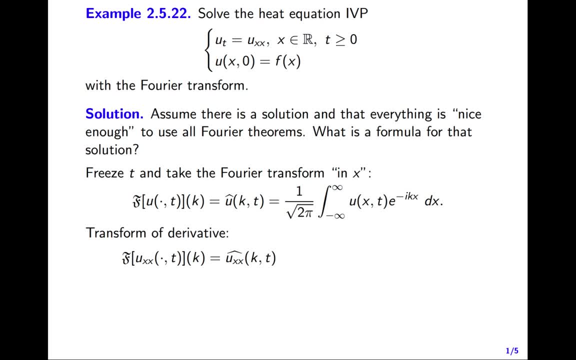 that's uxx hat of kt. So I'm taking two derivatives with respect to x. This is two derivatives. in the variable which I take, the Fourier transform. So I should get out an ik squared u hat of kt or a minus k squared u hat of kt. 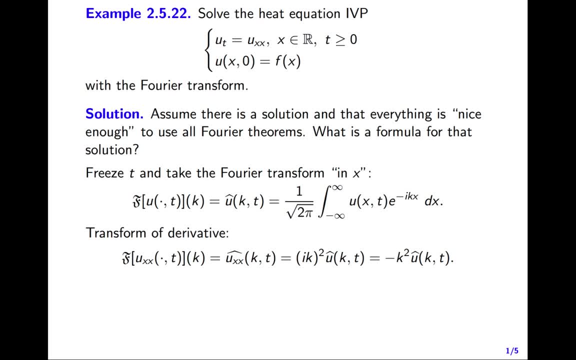 The important thing here is that the transform is occurring in the x slot and the derivatives are occurring in the x slot, which is why I get the ik each time I take an x derivative. On the other hand, in the heat equation I still have that u t derivative and I'm not 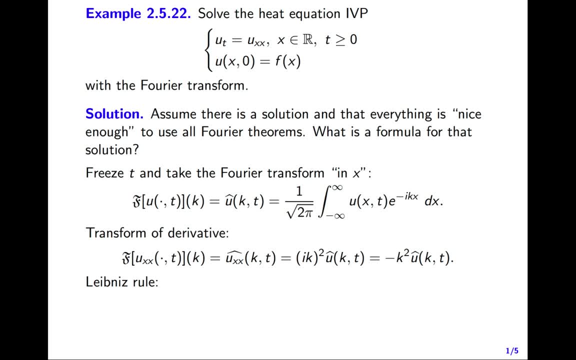 taking the transform with respect to t. So here I'll use the Leibniz rule: ut hat of kt. well, that's really defined to be equal to 1 over root, 2 pi, integral minus infinity to infinity. ut of xt, e to the minus ikx, dx. And what is that? Let's pop the t derivative outside the integral. 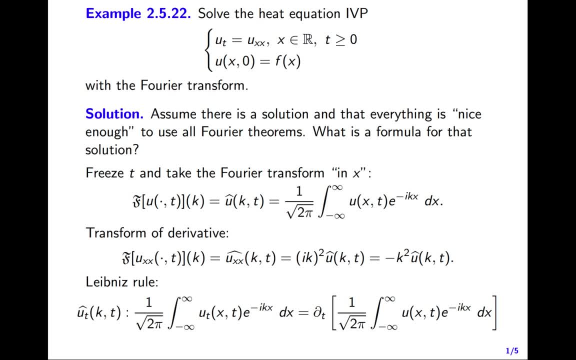 because I'm differentiating here with respect to t but integrating with respect to x. That is t derivative on 1 over root, 2 pi integral minus infinity to infinity u of xt e to the minus ikx. So that's t derivative on the Fourier transform of u, In other words, partial t on u hat. 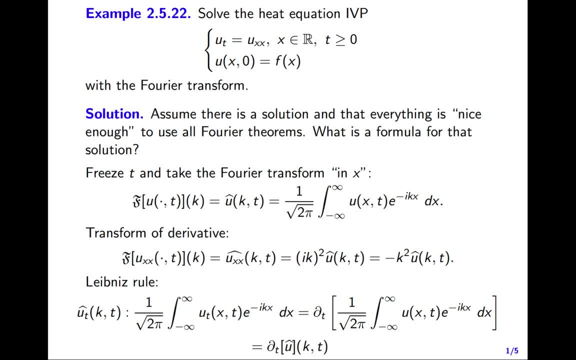 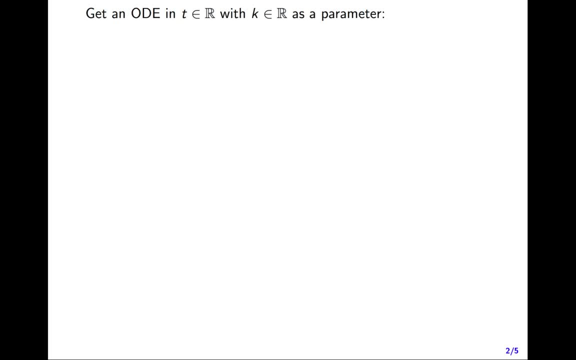 at kt. So what does this do? Taking the Fourier transform of the heat equation gives me now an ordinary differential equation in t with k as a parameter. So I have partial t on u hat of kt. equals ik squared on u hat of kt. 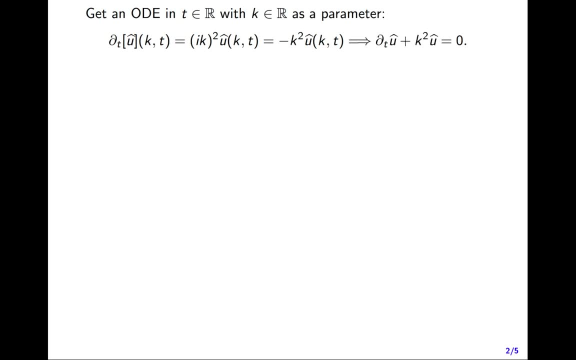 which is minus k squared u hat of kt. In other words, partial t on u hat plus k squared on u hat equals zero. So now, in this differential equation, what is moving and what is fixed? Derivatives are taken now with respect to time. t is the thing that moves. 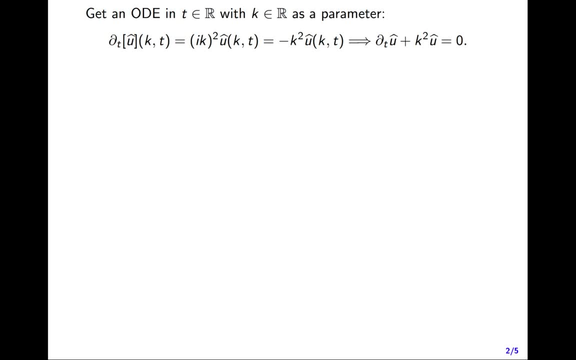 It is a real number, that is a parameter For each different real k. I get a different differential equation in the t variable. Now this differential equation, once we parse through all the notation, isn't that difficult to solve. t derivative on u hat plus a constant k squared on u hat equals zero. 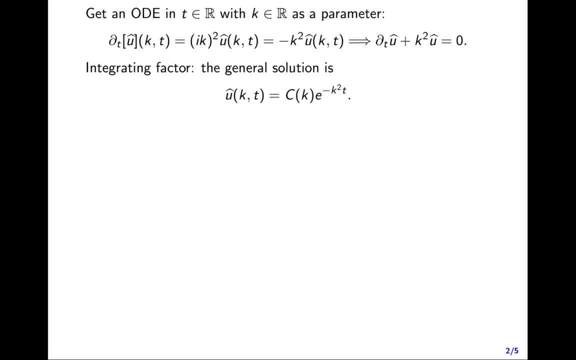 That means that u hat of kt is a constant c of k times e to the minus k squared t. And that's just the integrating factor method or separation of variables. Now remember your initial condition: We wanted u of x0 to be equal to f of x. 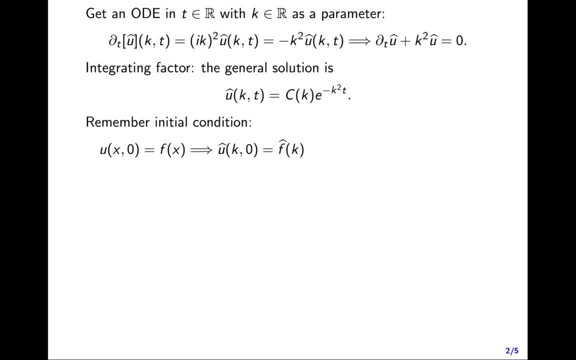 So I'm taking all my Fourier transforms and u This gives me: u hat of k0 equals f hat of k. So that tells me that the constant c of k, which is u hat of k0, has to be f hat of k. And so I can solve: u hat of kt equals f hat of k times e to the minus. 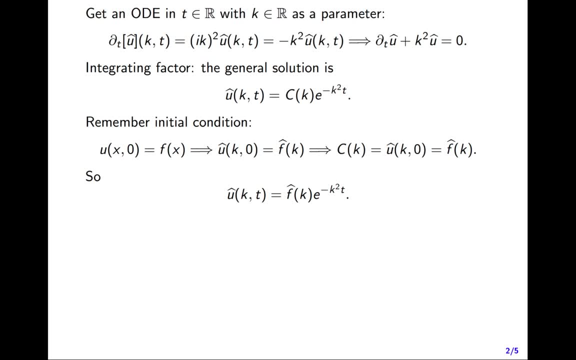 k squared t By the by. this is assuming that f is in L1.. That was one extra thing I have to put on my problem for this to work. So now I know what u hat of kt is and hopefully I can invert the transform and figure out what u is. Just to pause for a moment and 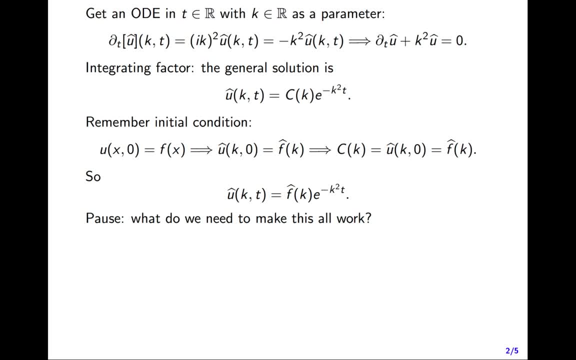 recap: what do I need to get all of this to work? Well, I was assuming that, for each t? u of dot, t was in L1, and so is ux, and so is uxx, and so is f. So, in order to take those, 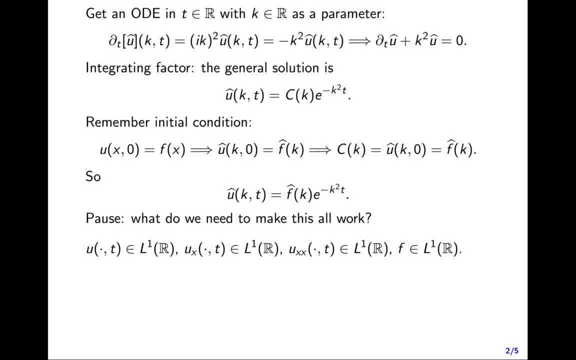 transforms. on the previous slide, whenever I froze t and just had a mapping depending on x, all those maps were in L1, and the temperature distribution f was in L1. And then I want to solve for u of xt. So I expect that u of xt is the inverse Fourier. 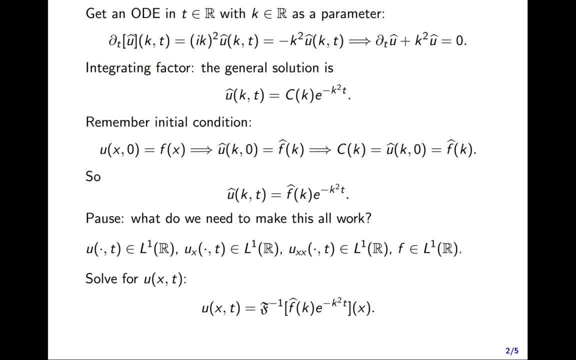 Transform with f hat of k times e to the minus k squared t at x, And again I'm taking the inverse Fourier Transform in the k variable. So t inside these square brackets is now reduced to a parameter. So you have to have a sort of dual vision here, Sometimes the time variable. 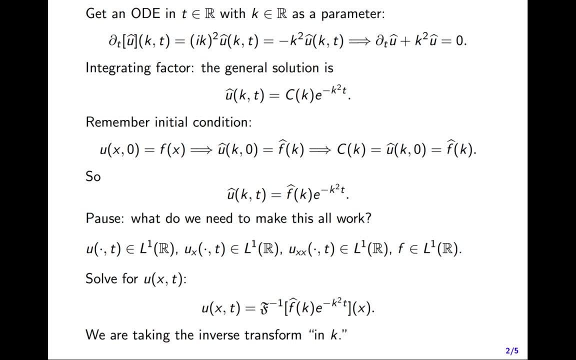 t is a parameter That's from the Fourier perspective, But then from the inverse Fourier, the differential equations perspective, time t still gets to move. So make sure you know what you're transforming with respect to and what you are differentiating with respect to. 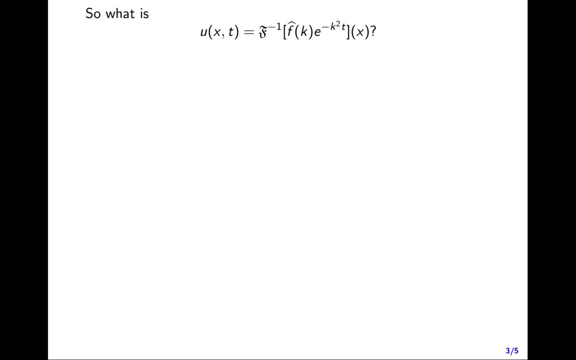 Okay, so what is u of? xt? equals inverse Fourier transform. f hat of k e to the minus k, squared t at x. How can I calculate this inverse Fourier transform? Can I do anything to it? Remember that, in general, the inverse transform of products is going to be the convolution of: 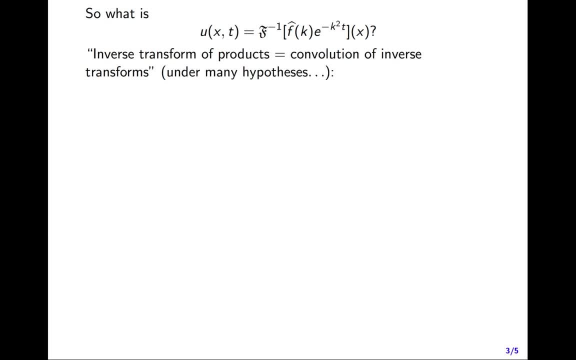 the inverse transforms under many hypotheses on everything involved. So what does this say? Inverse Fourier transform of f? hat of k times e to the minus k. squared t at x should be inverse Fourier transform of f? hat convolved with inverse Fourier transform of e to the minus k. 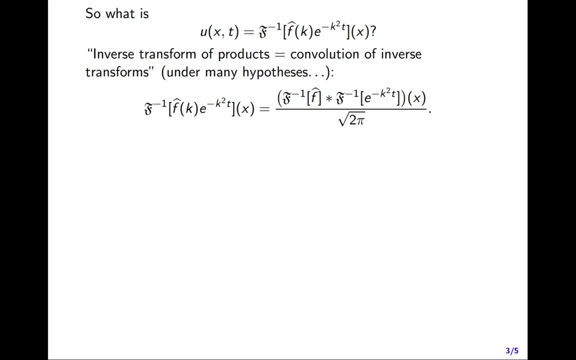 squared t at y, evaluated at x over root 2 pi. And this inverse Fourier transform of e to the minus k squared t. t is the parameter. k would be the variable of integration. So what's the inverse transform of the mapping? k goes to e to the minus k squared t. We can: 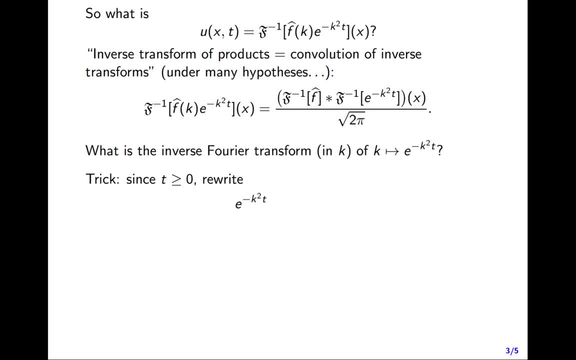 actually calculate this First time. t is greater than or equal to 0.. That's given at the start of the problem, So I can always rewrite this as e to the minus k squared t equals e to the minus root tk quantity squared. Easy enough, And now I'll define phi of big X to be e to the minus. 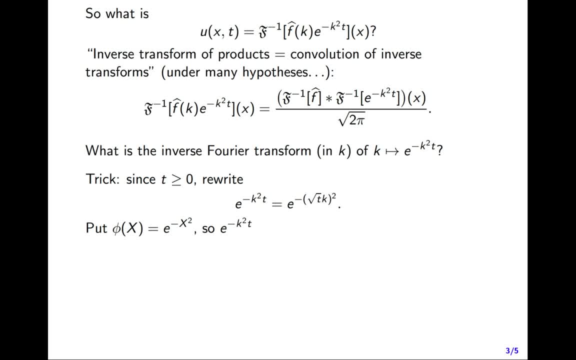 big X squared. So what does this say? e to the minus k squared, t is phi of root t times k. Now, phi is a function that's infinitely different And it's also in L1.. And we calculated in the past that phi hat of k is phi of k over 2 divided by 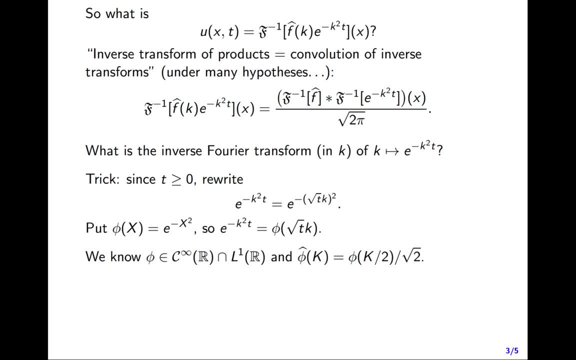 root 2.. This was a great calculation that we do in the notes and is very special about this: e to the minus x squared function. So the inverse Fourier transform of e to the minus k squared t at x is the inverse Fourier transform of e to the minus k squared t at x. 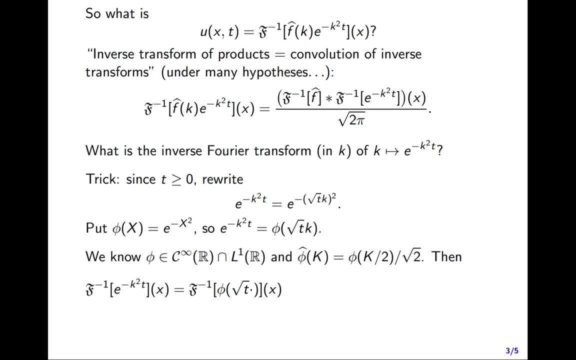 The inverse Fourier transform of phi scaled on the inside by root t. That's what phi of root t dot means And the inverse Fourier transform. I can also write that as a Fourier transform. So this is the Fourier transform of phi scaled on the inside by root t at minus x. You can go. 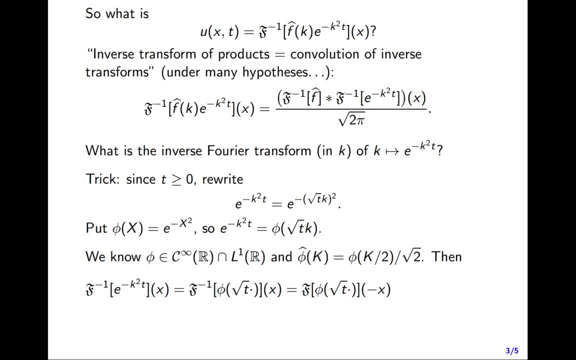 from the inverse transform to the regular transform by changing x to minus x. Scaling properties of the Fourier transform tell us that the inverse Fourier transform of phi scaled on the inside by root t. So the first sequence where the inverse Fourier transform is as a hometown of phi, squared infinite, should be seg. 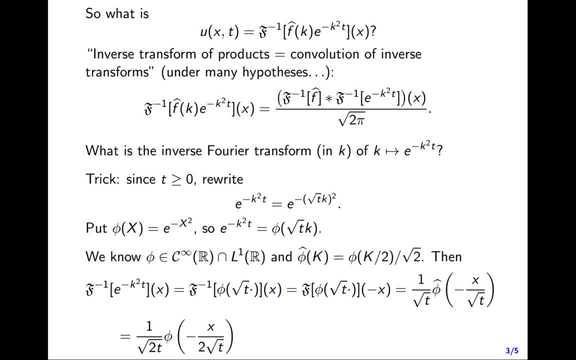 So we know that phi squared infinite is x squared simple executives. so we then need to break this all down to zero different pieces in a to everyone's name. So we have phi square plus τ squared times, k squared difficult, x squared square minus�1 over root t times. 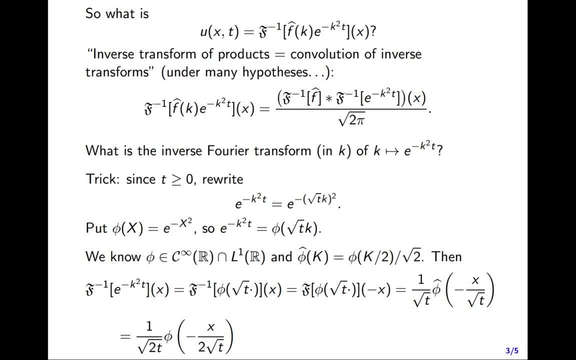 phi of minus x over 2 root t. So I popped the hat off phi and did some extra scalings. And then for my formula for phi, this is 1 over root 2 t e to the minus x squared over 4 t, again assuming that t is positive. Okay, that was quite a calculation. This might be a. 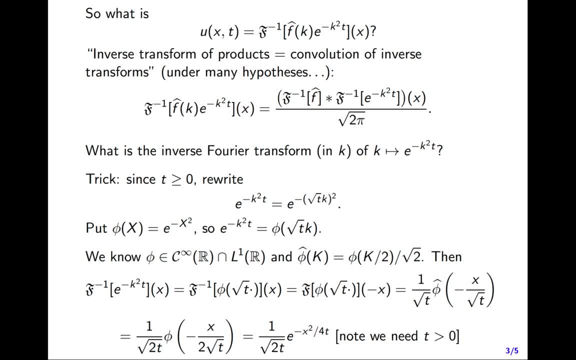 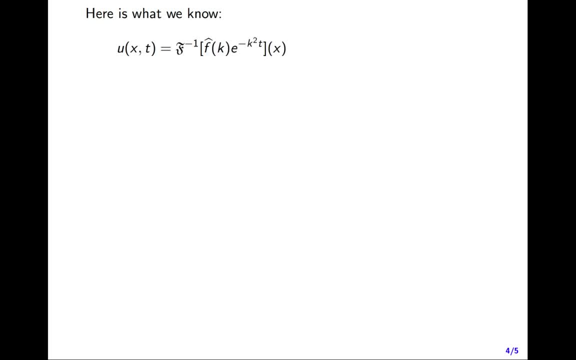 moment to hit pause and make sure you can go through all of it. And so here's what we get: u of x. t is the inverse Fourier transform of f hat of k times e to the minus k squared t at x, which, by convolution, is the inverse Fourier transform of f hat. convolved with inverse. 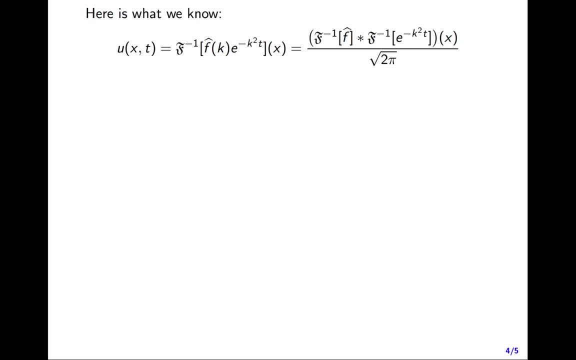 Fourier transform of e to the minus k squared t at x over root 2 pi. And we know that the inverse Fourier transform is: the inverse Fourier transform of e to the minus k squared t over root 2 pi. The inverse Fourier transform of e to the minus k squared t at x. 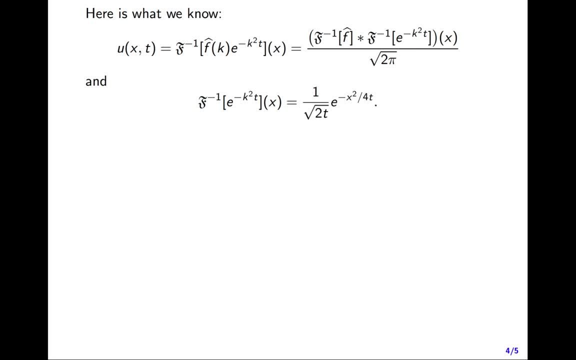 is 1 over root 2 t, e to the minus x squared over 4 t, assuming t is positive. And we also want for this function, f, that the inverse Fourier transform on f hat should be f. So what do we really need about f? We need f to be in L1 and continuous and piecewise. 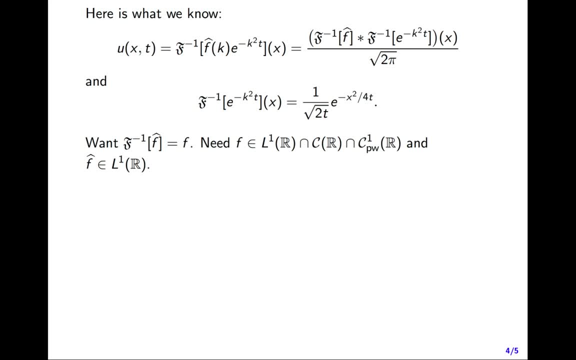 continuously differentiable and we need f hat to be in L1.. So if we assume all this about our initial temperature distribution, then nice things are going to happen, Namely the inverse Fourier transform of f hat. convolved with the inverse Fourier transform. 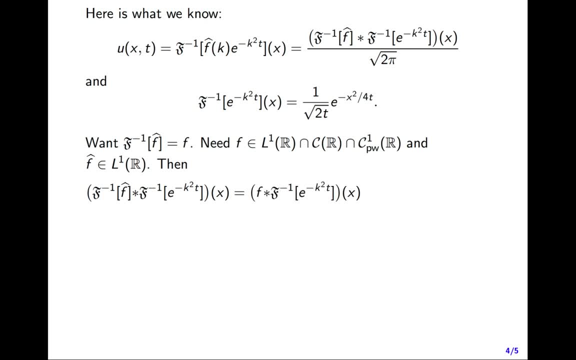 of e to the minus k squared t at x will turn out to be f convolved with the inverse Fourier transform of e to the minus k squared t at x. And because convolution is commutative, I could just write that as inverse Fourier transform of e to the minus k squared t at x. 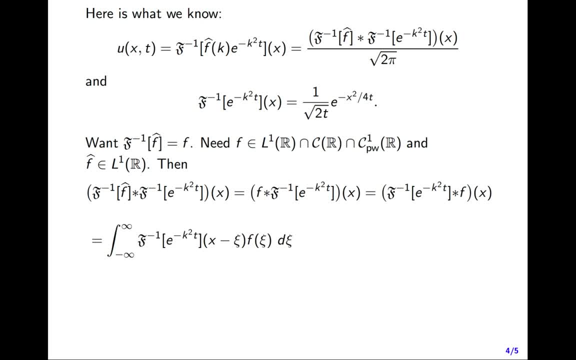 the minus k squared t convolved with f. and if i go into the definition of the convolution, that's the integral, from minus infinity to infinity, inverse Fourier transform of e to the minus k squared t at x minus xi times f of xi, where i'm integrating with respect to xi. and then, if i use 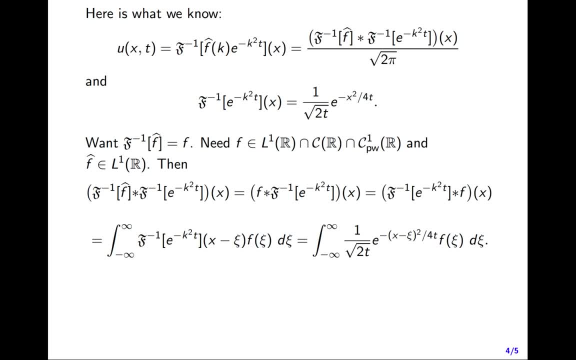 my definition of this inverse Fourier transform of e to the minus k squared t. this becomes integral, minus infinity to infinity, 1 over root t. e to the minus x, minus xi quantity squared over 4 t times f of xi. so all together, incorporating a few extra factors of pi? u of x, t is 1 over root 4 pi t. 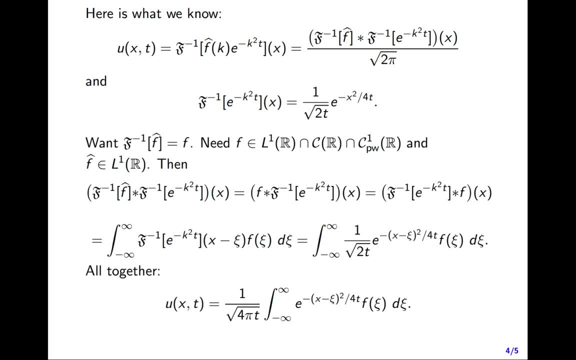 integral minus infinity to infinity, e to the minus x minus xi, squared over 4 t f of xi. okay, another good time to hit pause and make sure you can chase through all these calculations. big picture: we used convolution, we used some Fourier theory, some inverse Fourier theory. 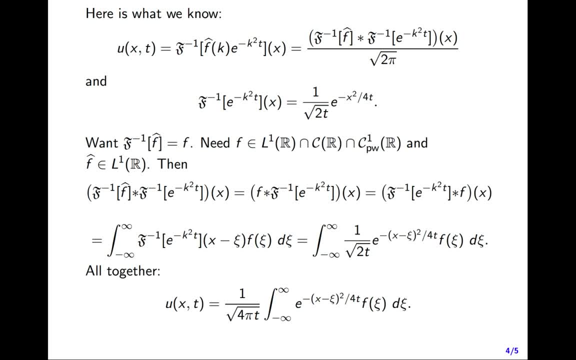 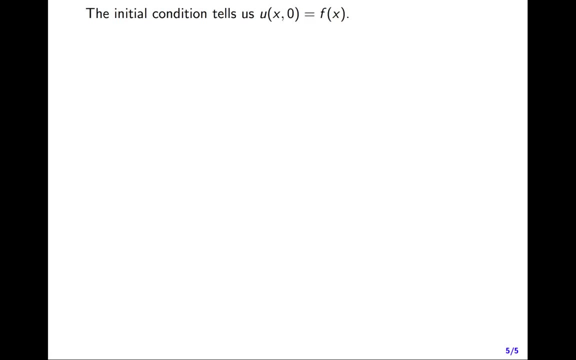 and we used a special Fourier- transform identity- that we proved elsewhere, and then we just convolved with the definition and simplified things as far as we can go. now again, we should watch out. we are demanding here that we hope we get the initial condition for the problem. u of x: 0 is equal to f of x. 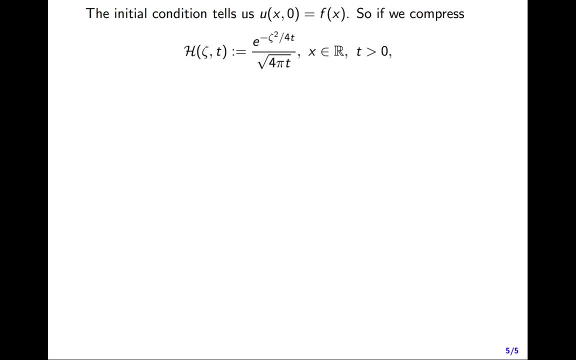 if we have any conditions for this problem, then we know that when t is positive, what happens? when t equals zero, then we know what happens. we have an initial condition for the problem: u of x- 0 is equal to f of x. so let's compress our notation a little. let's put: 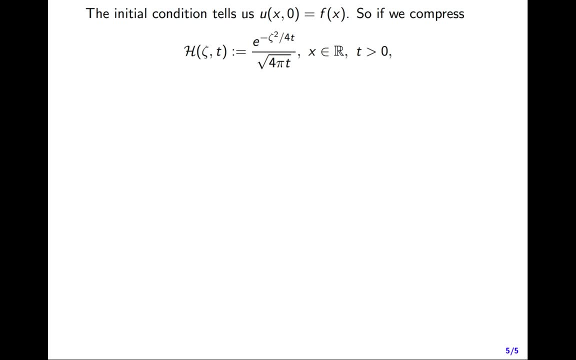 h of zeta t to be e to the minus zeta squared over four t. whole thing divided by root 4 pi t. u is h of dot t convolved with f at x for all real x and t positive, and f of x for all real x and t equals 0. 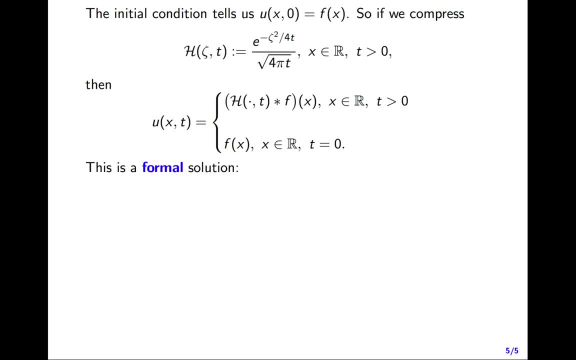 By h of dot t convolved with f. this is my notation of replacing the variable, which I'm convolving by a dot. so this is convolving in the zeta slot of h, as on the previous slide, And this is a formal solution. What do I mean by this? 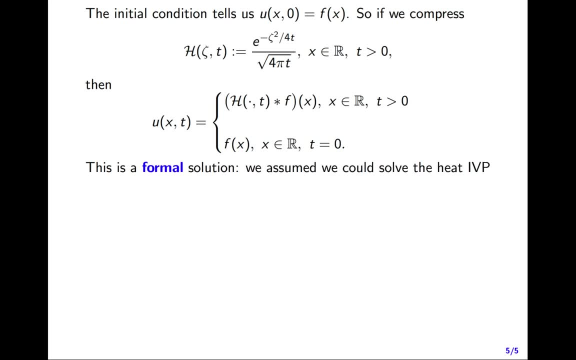 We assumed that we could solve the heat initial value problem and that u and f were nice enough for all the Fourier theory to work, And that u and f were nice enough for all the Fourier theory to work And we got this convolution solution. 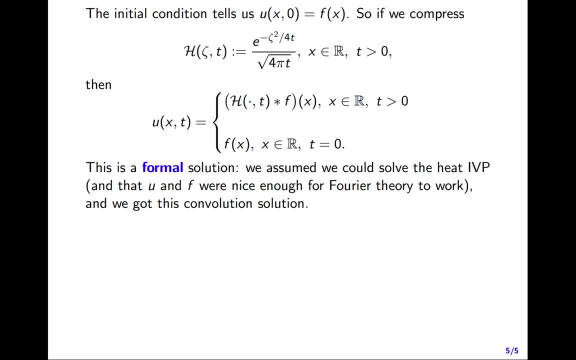 So if f satisfies all the properties on the previous slide, then we should be able to define a function u of x, t as this piecewise function, In particular the convolution, will be defined. Then we have to check that this actually solves the partial differential equation. 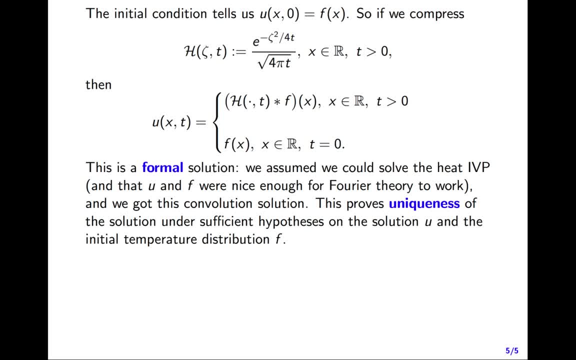 We've shown, you might say, uniqueness of the solution under sufficient hypotheses on u and f for us to use the Fourier transform and that the initial temperature distribution f is nice. But with this piecewise formula, is u continuous? Is it differentiable? 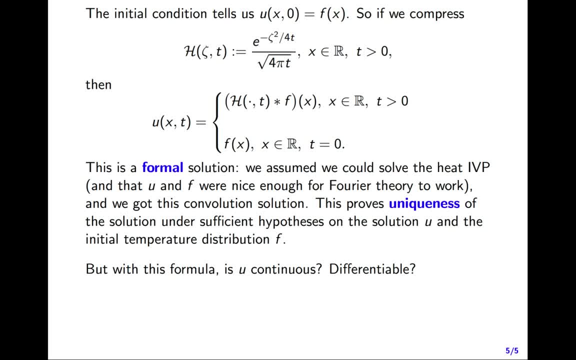 It's always what we should ask ourselves when we have the piecewise formula, and always what we should ask ourselves if we have a formula given by a Fourier transform or a Fourier series. Do we actually have ut equals uxx? And to check all that we would need to do some calculus. 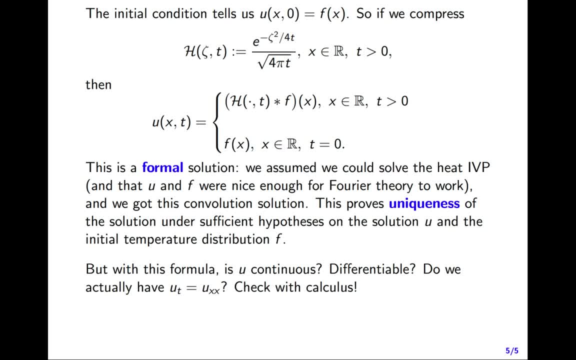 and grind through differentiating the convolution, dealing with this awkward jump or piecewise condition from t equals 0 to t positive, and it would be a lot of calculus using Fourier theory along the way. We will not do that. We will be content with having this as a formal solution. 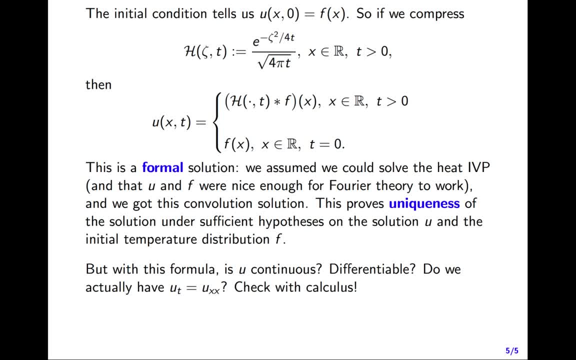 But trust me that it does work out that this function u is continuous and sufficiently differentiable and solves the heat equation. Last thing: Sometimes people call the function a or zeta t the heat kernel or the fundamental solution of the heat equation.